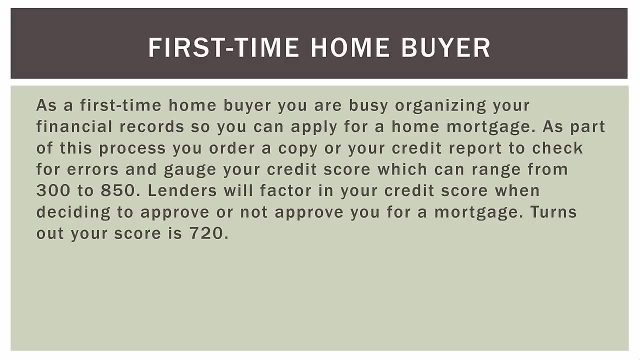 order a copy of your credit report to check for errors and gauge your credit score, which can range, at least here in the US, from 300 to 850.. Now lenders will factor in your credit score when deciding to approve or not approve you for a mortgage. Now they will. 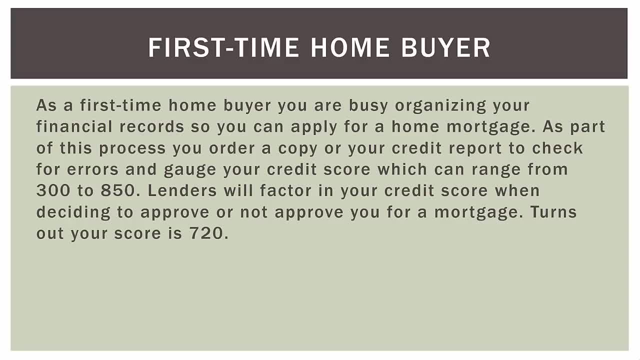 factor in other things like your income, how long you've been at your job and other things, But your credit score is definitely an important part of their decision. Now it turns out your credit score is 720 on that scale of 300 to 850. 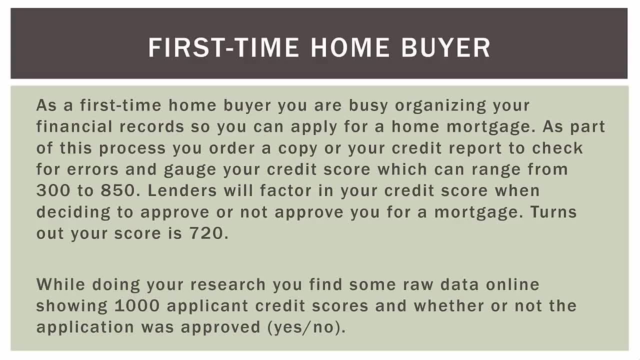 Now, while doing your research, which you are dutifully doing as a potential homebuyer, you find some raw data online, So there's data floating around the web everywhere. So you are lucky enough to come across this data set that has 1,000 applicant credit scores and whether or not 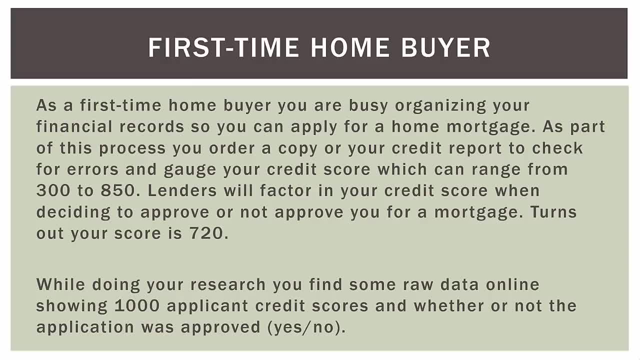 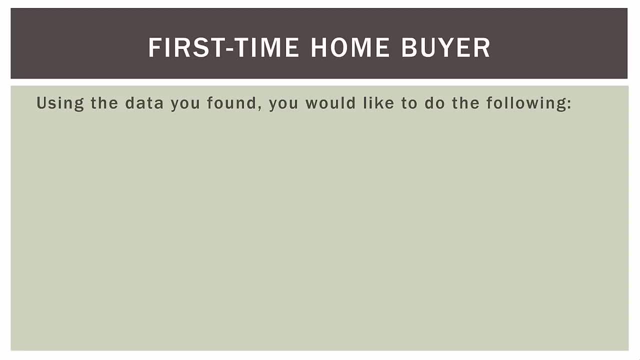 the application was approved. so yes or no for the home mortgage? Yup, back to our math Bowdoin error and give it another look at this formula. So that's scale. Now, you most likely won't believe this, but I did. 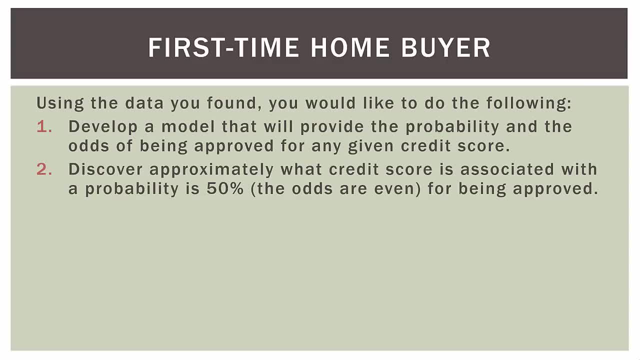 Now, using the data you found, you would like to do the following. Number one: develop a model that will provide the probability and the odds of being approved, for being approved. So if I walk into the bank with a certain credit score, it's basically like flipping a coin. 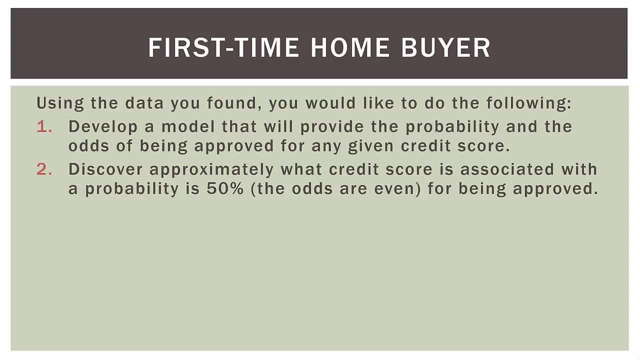 My probability is 50% of being approved, which is the same way of saying the odds are even. We wanna know what credit score that is on our scale. Number three, input your score of 720 into the model to determine the probability and the odds. 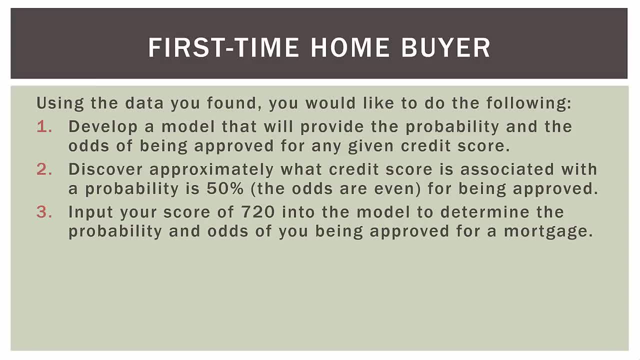 of you being approved for a mortgage, which, of course, is very important to you- And finally determine how improving your credit score from 720 to 750 would affect your probability and odds for being approved for the mortgage. So let's say your score is 720, you find that out. 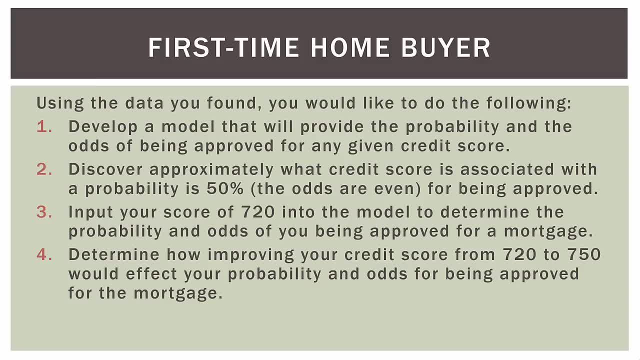 So you're gonna wait a little bit and see if you can get your credit score a bit higher- up to 750, by paying down some debt. Maybe you know that you're gonna get a promotion and a higher salary sometime soon, or something like that. 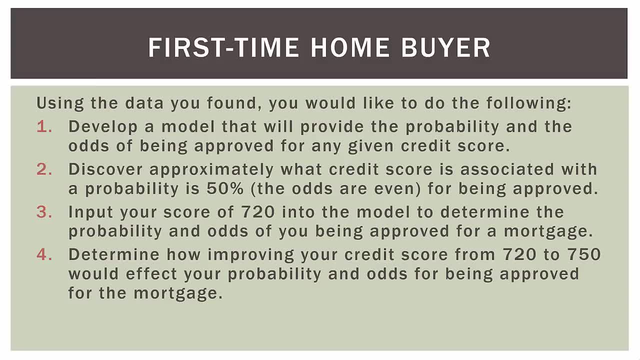 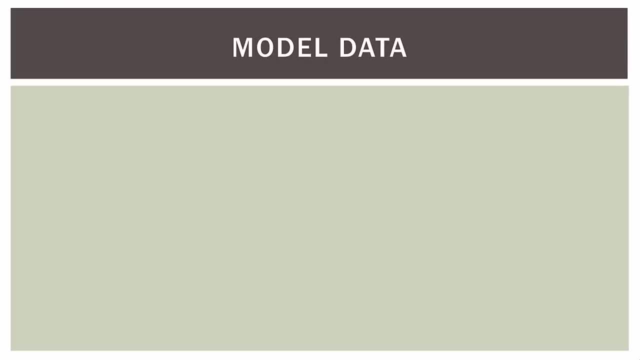 and you think that your score may improve And you wanna know how that improvement in your score would affect your probability and odds of being approved for the mortgage. So here is just a little chunk of that 1,000 observation data set. So there are only 15 here. 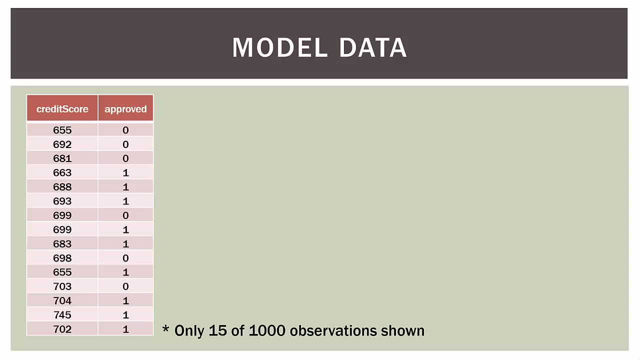 but I just wanted you to see how it's organized. So we have the credit score on the left and approved on the right. So again, the N is 1,000.. The credit score is the applicant's credit score, from 300 all the way up to 850. 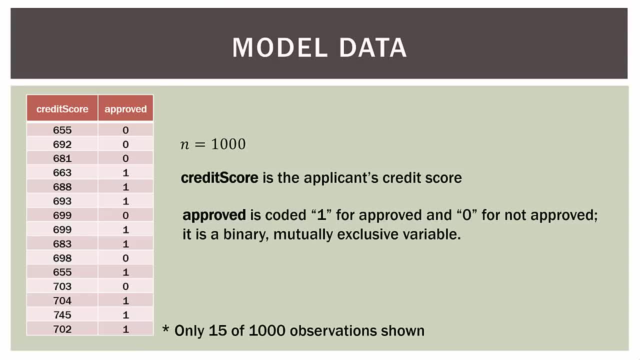 It is coded as a one for approved and zero for not approved, So it is binary, It is a dichotomous variable and it is mutually exclusive. So you're either approved or you're not approved. There's no in between. 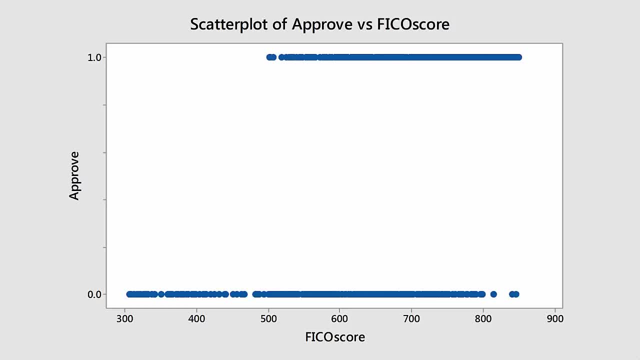 Now, as a good analyst and a good stat student, or whatever it is you might be, you create a scatter plot of your 1,000 observations, But it looks like this: Now, what is this? So, if you look on the left-hand side, 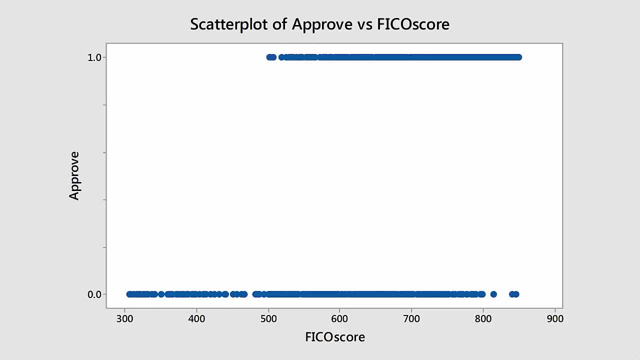 we have approve and we have zero at the bottom, So that means the application was not approved, And at the top we have a one, So that means the application was approved. But we have the data points in two lines, So the credit score along the bottom. 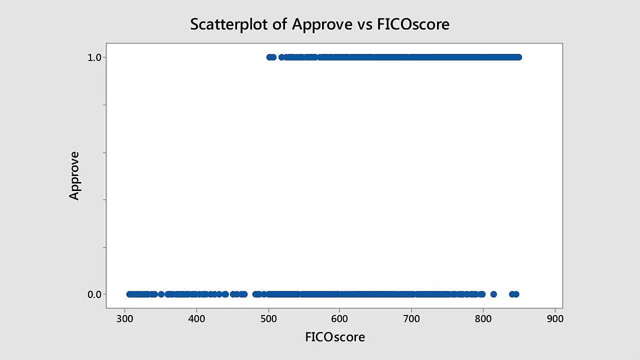 so FICO score is just a certain type of credit score that's widely used. So if the dot is on the bottom, that means for whatever credit score that was, the application was not approved. If it's at the top, it means it was approved. 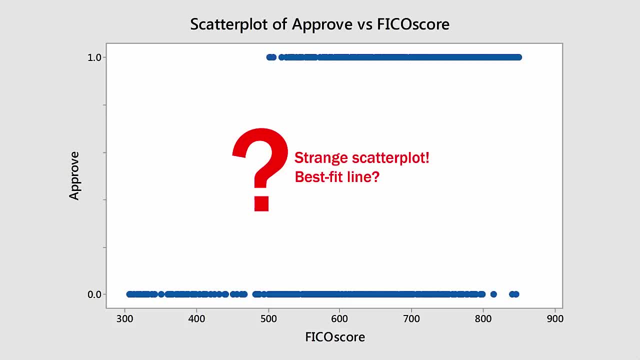 Now, how can we put a best fit regression line on a scatter plot that looks like this? It doesn't make any sense to do it how we would usually do it in normal linear regression, So obviously we're going to come up with some other technique. 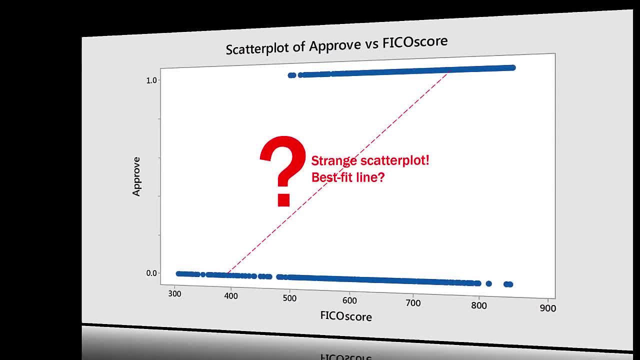 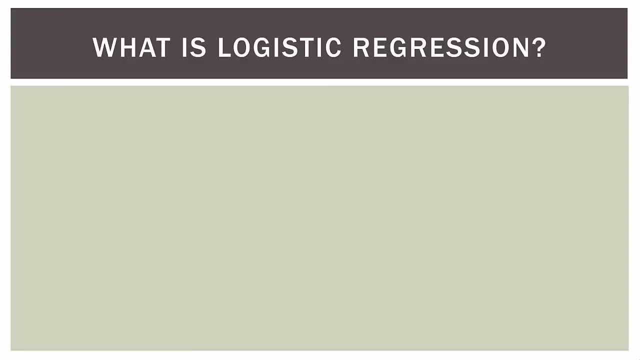 and that's what logistic regression allows us to do. Now that we have set the stage with the problem, we're going to look at. what is logistic regression Now? logistic regression seeks to do the following, Among other things: It seeks to model the probability of an event occurring. 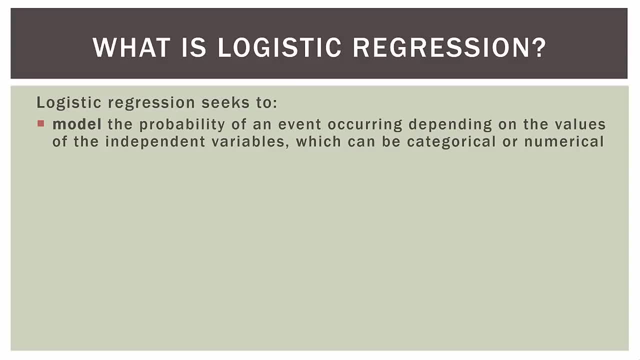 depending on the values of the independent variables, In this case credit score, which can be categorical or numerical. So model the probability of an event occurring depending on the other independent variables. It seeks to estimate the probability that an event occurs for a randomly selected observation. 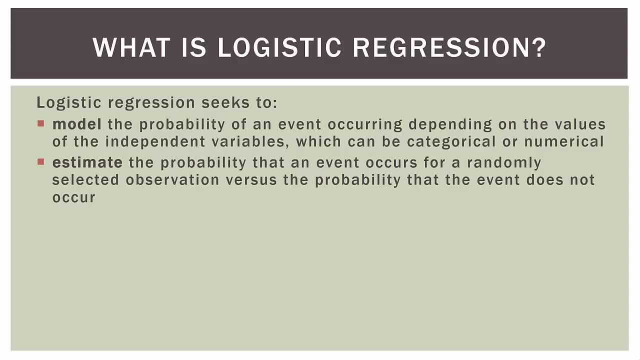 versus the probability that the event does not occur. So for a random observation in the data or some other observation that we want to predict, we want to estimate the probability that the event occurs versus that it does not occur. It seeks to predict the effect. 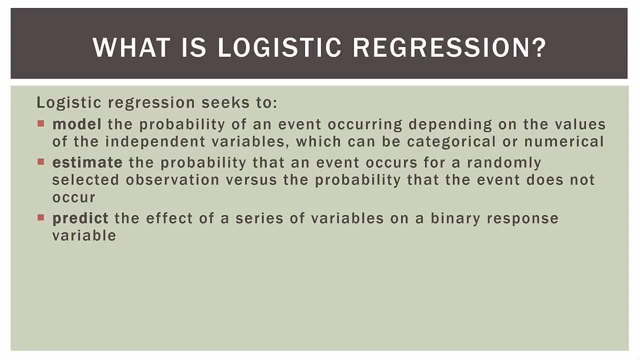 of a series of variables on a binary response variable. So in this case we only have one independent variable, credit score, but we can have more. so logistic regression can work a lot like multiple regression with several independent variables and the one dependent variable that is binary. 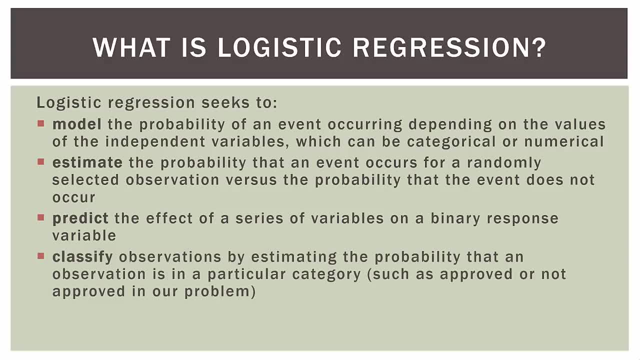 so zero or one. We can also seek to classify observations by estimating the probability that an observation is in a particular category. In this case, the applicant is either in the approved category or they're in the not approved category, So we can classify observations. 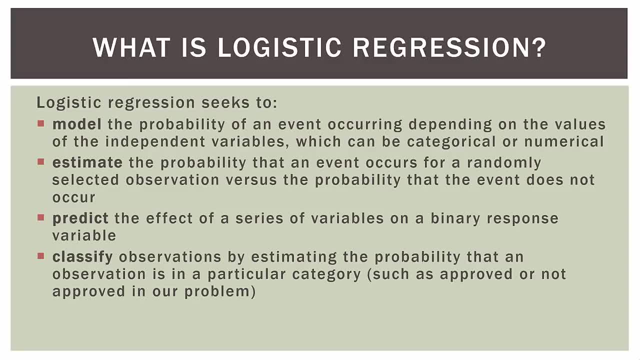 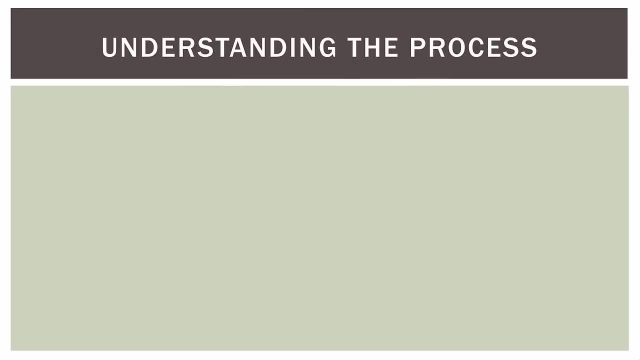 So model, estimate, predict and classify. So let's try to understand and visualize the problem we're working with. So in this case we have a bunch of credit scores. So an applicant walks into the bank and they have some sort of credit score. 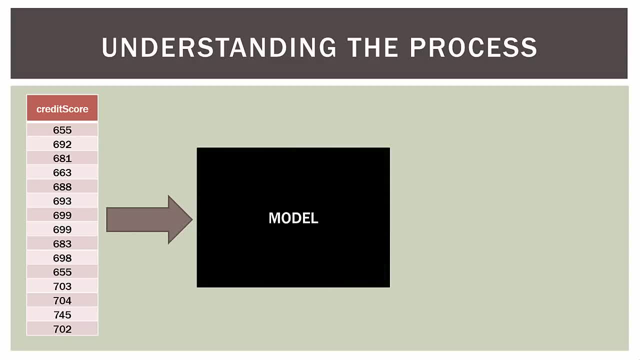 Now the bank or other lending institution feeds that into their lending model. Their credit score goes into the model and then when it comes out, it's either approved or it's not approved. So this black box in the middle is what we're trying to understand. 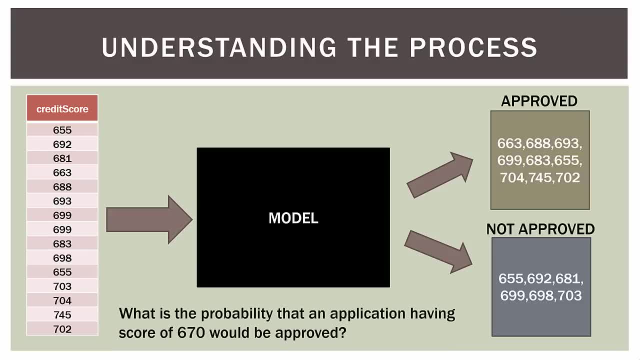 So we could ask what is the probability that an application having a credit score of 670 would be approved, So it would end up in the approved category up here on the top. So credit scores get put into some model, a decision model by the bank or other lender. 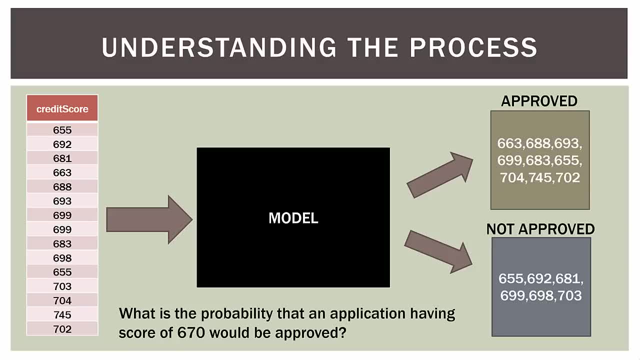 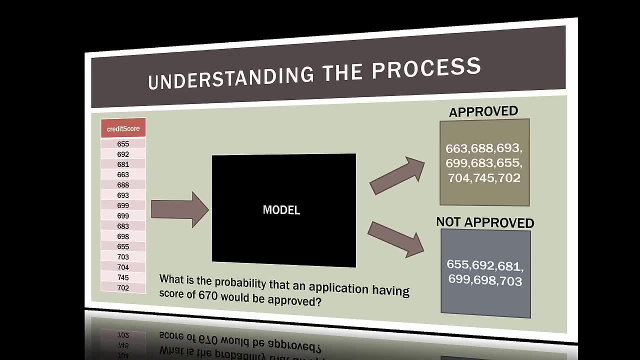 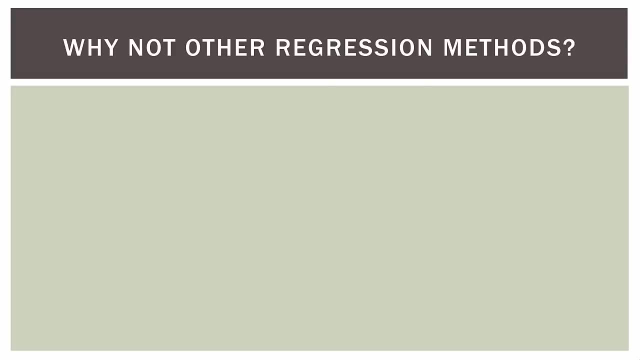 and then the bank or the lender puts that application into the approved or not approved category. That's basically what we're trying to model in this logistic regression problem. Now I am kind of making the assumption that if you're studying logistic regression, you have to some extent studied simple linear regression. 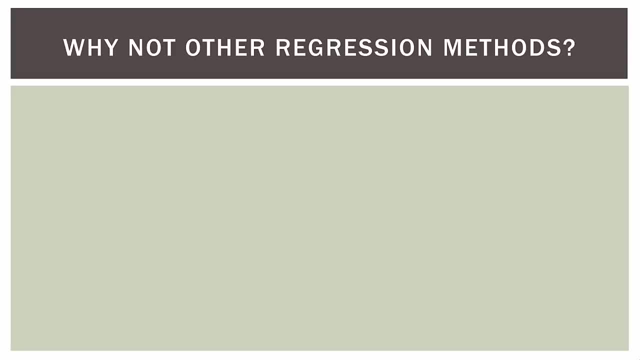 and multiple regression. Now, if you've studied those, you might have a very good question: Why can I use one of those for this type of problem? Well, here's why. Number one, simple linear regression, is one quantitative variable predicting another quantitative variable. 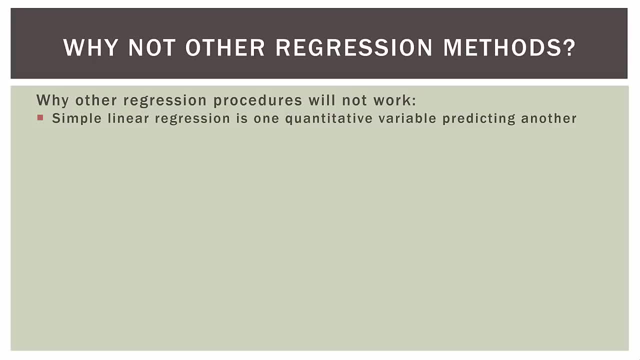 Now, in this case we have a dichotomous dependent variable. So approve or not, approve is one or zero. That's not a quantitative variable. Now, multiple regression is just simple regression with more independent variables. So those are basically the same type of problem. 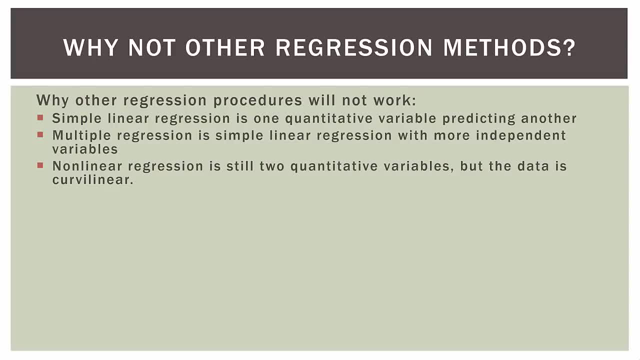 Now we have nonlinear regression. That's still two quantitative variables but the data is curvilinear. Now if we ignored those warnings, running a typical linear regression in the same way on this type of data has some major problems. Now, binary data in this case. approve or not approve. 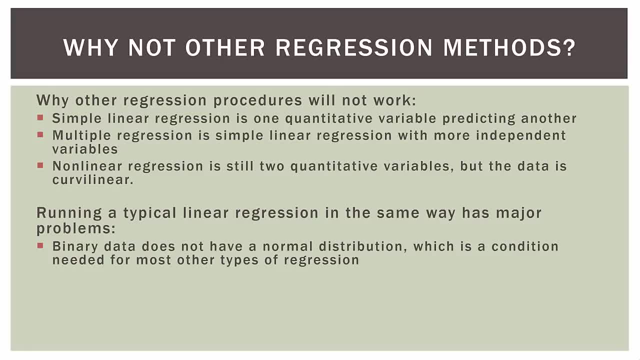 does not have a normal distribution and you could see that by looking at the scatter plot, which is a condition needed for most other types of regression. The predicted values of the dependent variable can be beyond zero and one in those other types of data. 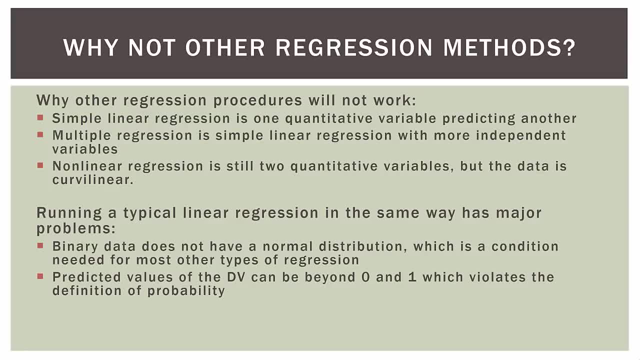 So that's a good thing. So remember, in logistic regression we're dealing with probabilities And the rule of probability is that it has to be between zero and one. If we use the other types of regression, the values can be beyond zero and one. 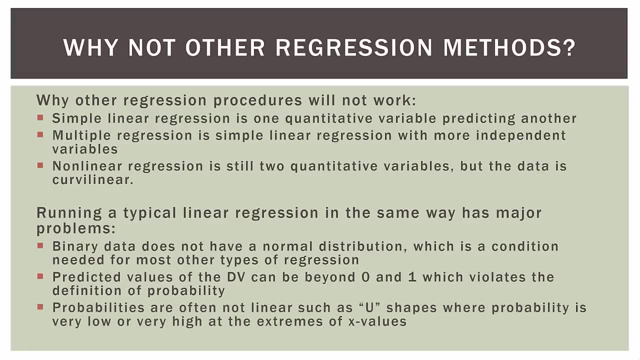 which obviously is not going to work, And probabilities are often not linear, such as U-shapes where the probability is very low or very high at the extremes of the X values. So you can probably think of different examples, So one example could be the probability. of contracting the flu. So the probability of getting the flu is higher. if you're younger, so a baby or an infant or toddler, and if you're older, so say in your 60s, 70s and 80s. 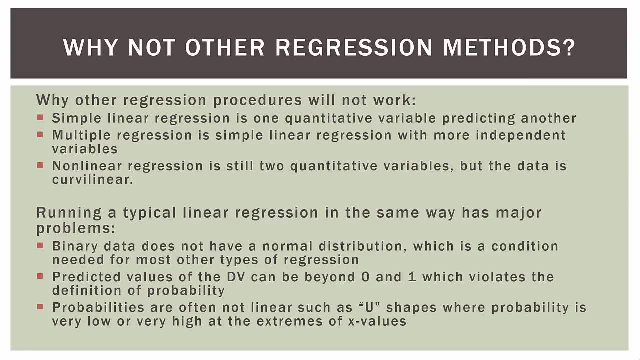 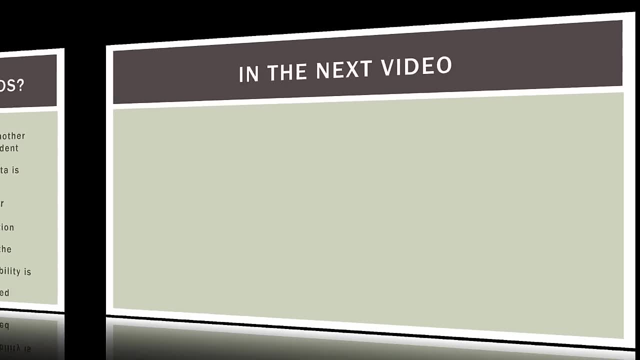 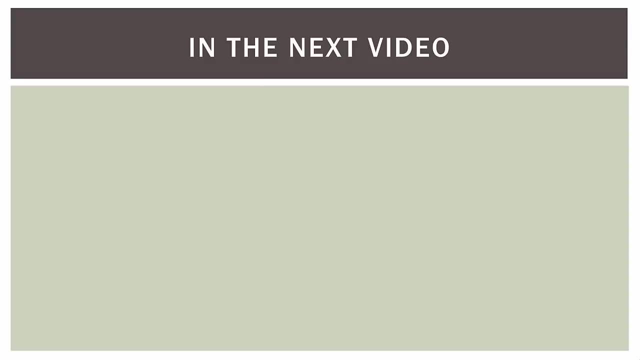 So the probability is higher in the extremes than it is in the middle. So probabilities often have different shapes in their distribution along the X variables. So now that we have set the stage by introducing our problem and going over the basic conceptual foundation of what logistic regression is, 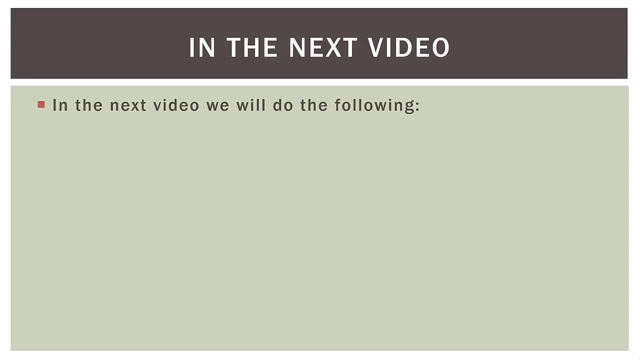 let's talk about where we're going in the next video. So in the next video we will do the following: We will review basic probability, So we won't go into much depth, We'll just go over the basics because, obviously, understanding probability